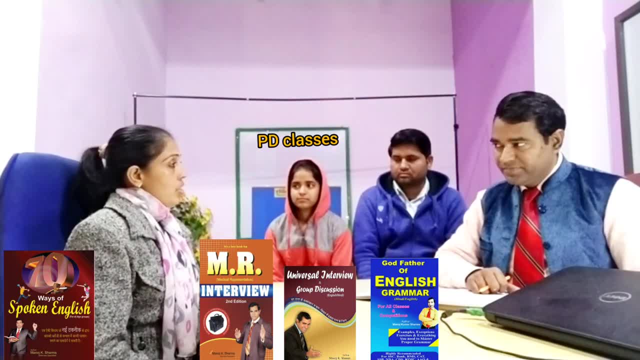 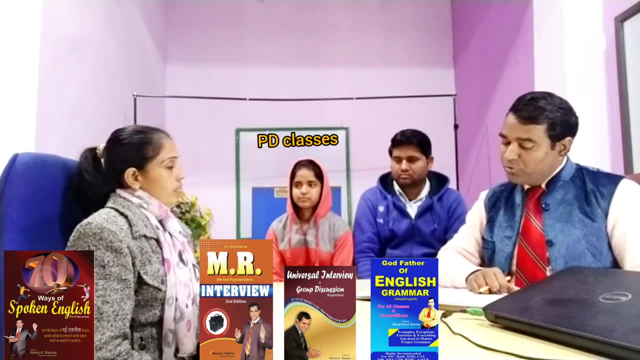 Yes, sir, Pythagoras. triplet means three positive integers are in the form of like: a square plus b square equals to c square. Okay, How could you explain this? How could you identify hypotenuse in a right angle triangle? Yes, sir, Sure, Hypotenuse. 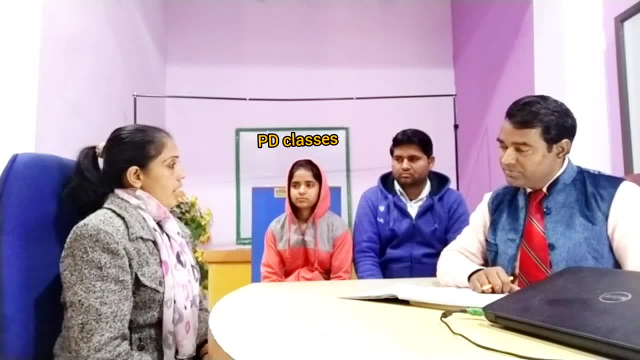 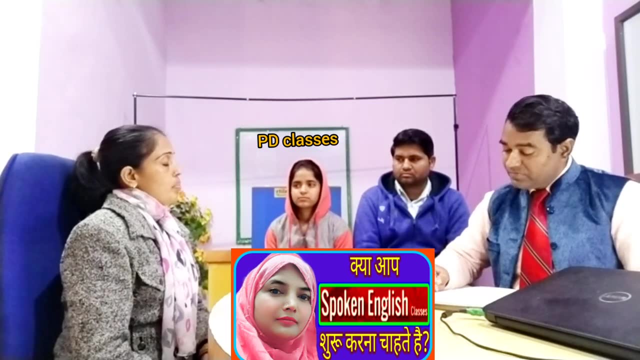 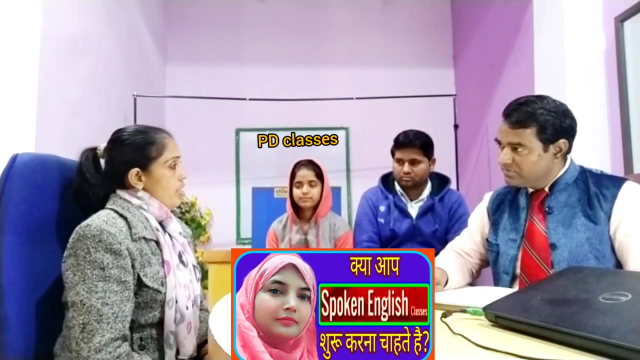 in a right angle triangle is the highest, longest side. Okay, Can you tell me the relation between sine theta and cos theta? Yes, sir, Sine square theta plus cos square theta is always 1.. And in form of tan theta, sine theta upon cos theta equals to tan theta. Okay, Why you opted? 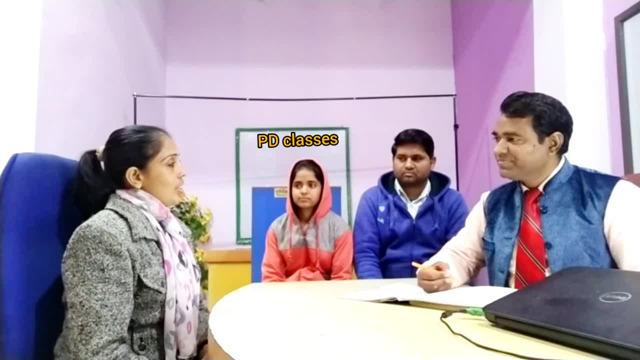 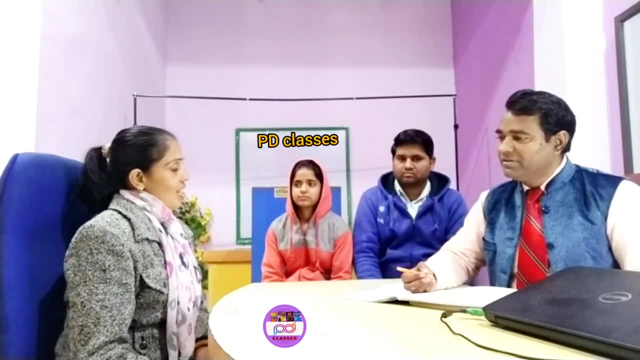 mass as your career. What is the reason, Sir? mass is an interesting subject, Okay, And so I think I can choose. No, I agree with you, It is very interesting. But what other factors motivate you to join mathematics teaching? Yes, sir, My family member, my class. 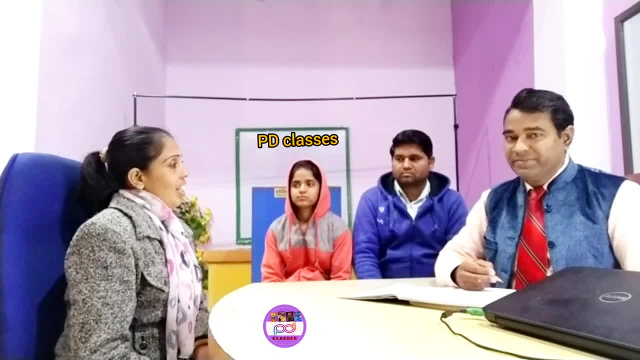 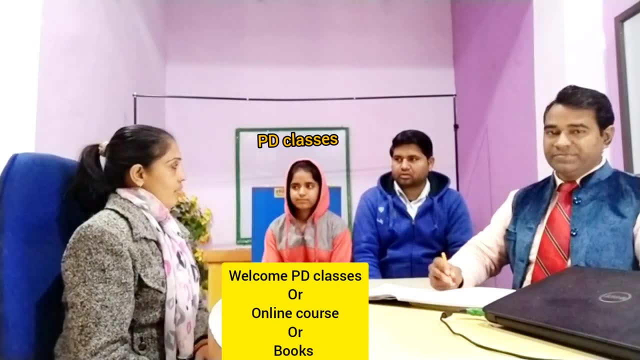 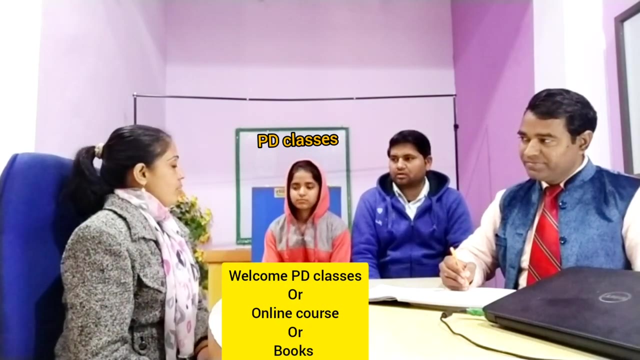 teachers when I got highest marks in the subject and showing my interest. so I choose: Okay, Yes, please, Mr Anand, you can have your questions. So, ma'am, you tell me area of circle: Area of circle is pi r square. You tell me surface area of circle is pi r square. 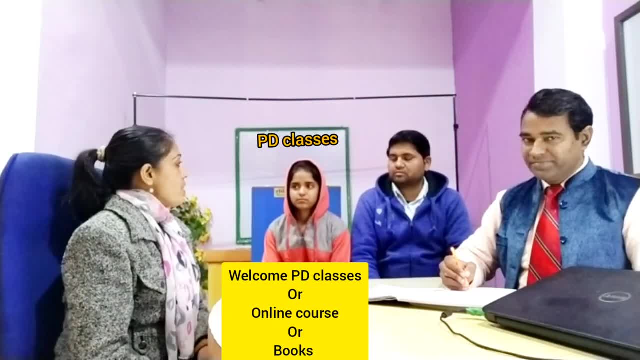 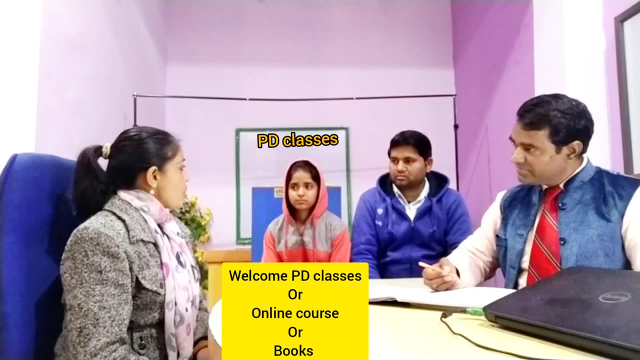 Of cuboid. Yes, sir, Surface of surface area of cuboid is equals to 2 multiplied by lb plus bh plus hr. Fraction, Fraction: Fraction is in the form of numerator divided by denominator. Fractions are many types, like proper fraction, improper fraction and mixed fraction. In proper 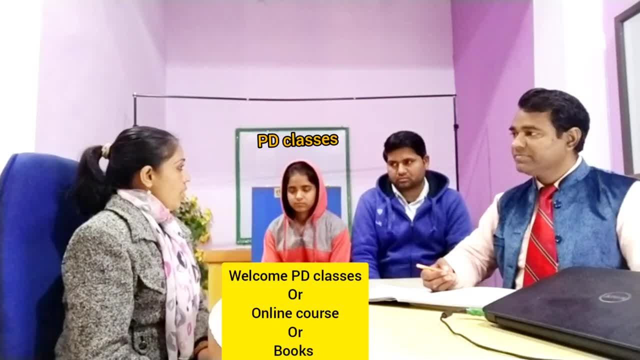 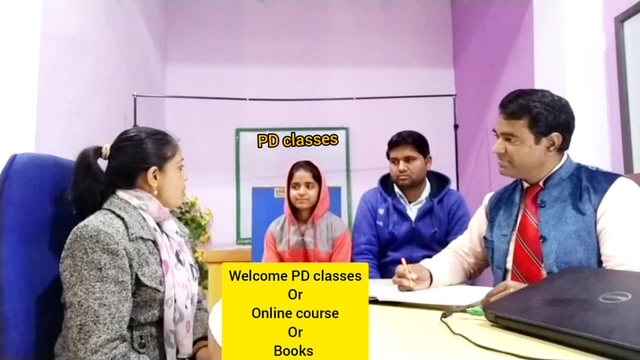 fraction numerator is always smaller than denominator, like 1 by 2.. And in improper fraction, numerator is always greater than denominator, like 3.. 3 by 4.. And mixed fraction is in a whole than half part, like 3, 1 by 2.. 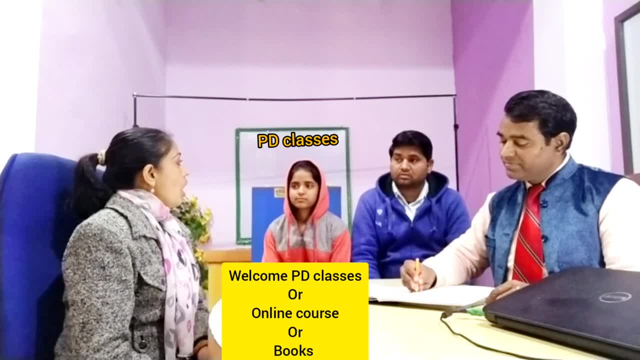 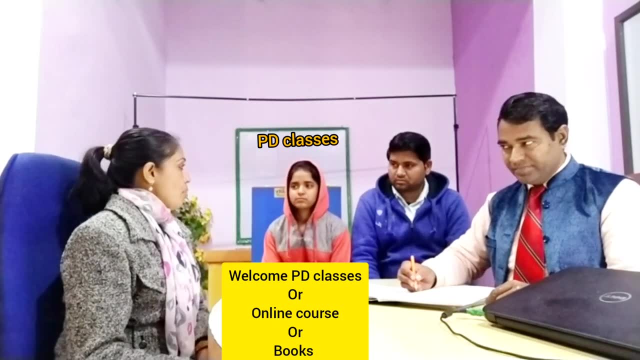 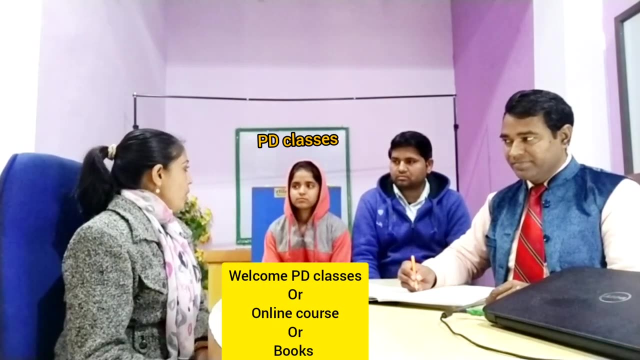 Okay, Like fraction and unlike fraction. Yes, sir, Like fraction are these type of fraction, which is in which denominators are same, like 1 by 2, 4 by 8 and 16 by 32.. And unlike fractions in which denominator and numerator are both different in different. 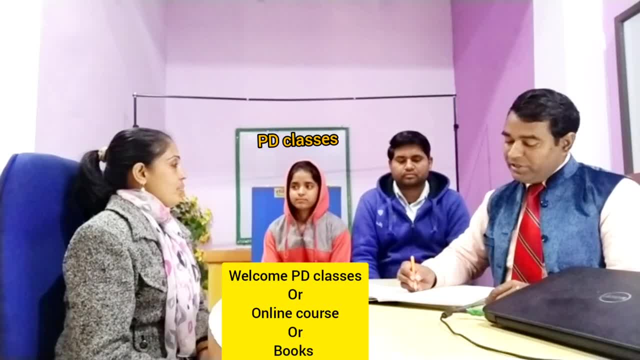 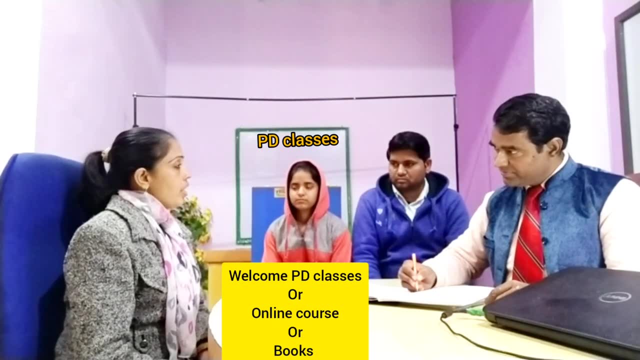 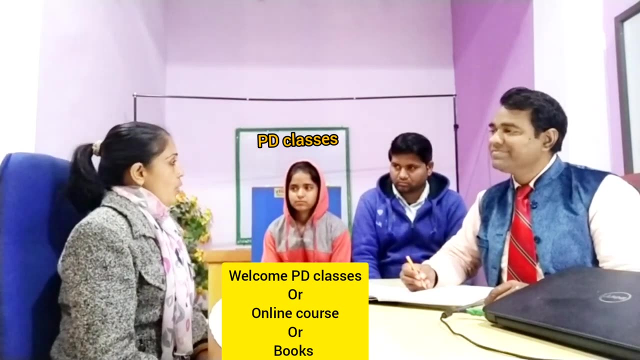 terms? Yes, Okay, What is the value of pi in fraction, Fraction or decimal form? Yes, sir, Pi. the value of pi in fraction form is 22 by 7 and in fraction form, 3.14.. Okay, Please introduce yourself. Yes, sir, My name is Ritu Raj which. means beauty and love, And I am very much similar to my name, as I am a cheerful and philanthropist personality. I belong to Bikaner, and which is famous for its various fort and and, like Junagadh, Ghazni Palace and Lalgarh Palace are one of them. I have done my great. 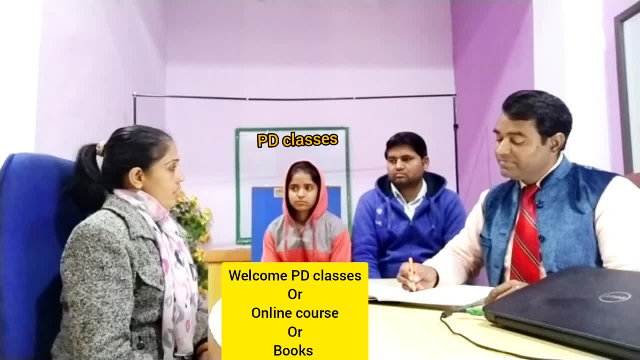 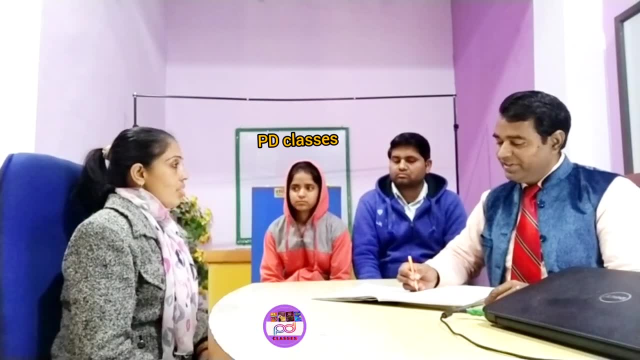 graduation from Bikaner University and BA from Rajasthan University, Jaipur. I have a solid experience of teaching, specially in maths and English- at least 10 years. Very good. I like to meet positive attitude, personality and exploring new ideas and culture and learning. 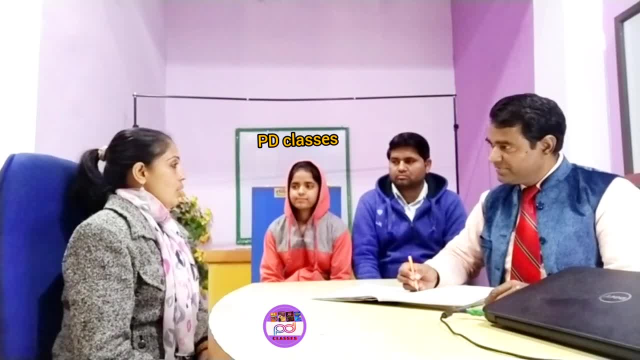 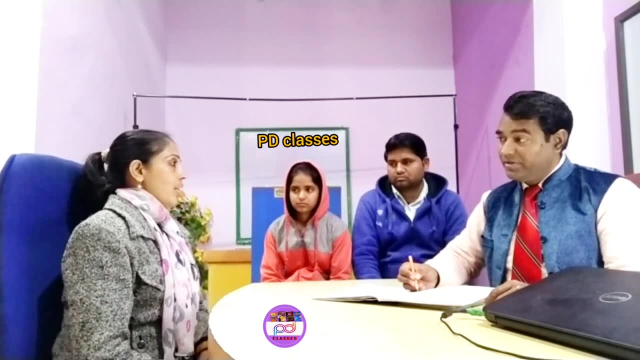 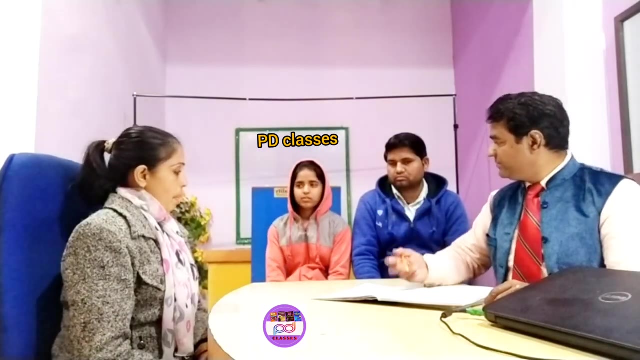 more of them about them. I am a versatile girl because of my adjustable nature. I am a team spirit girl- I don't try to hog all the credit- and I am a creative girl. I am a strong girl. It is my strength, Okay, So, Mukta, you can have your question, please. 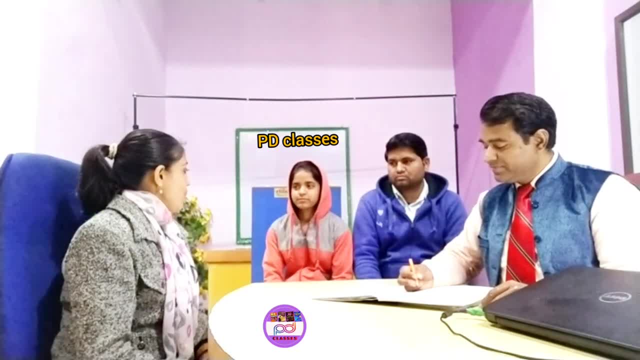 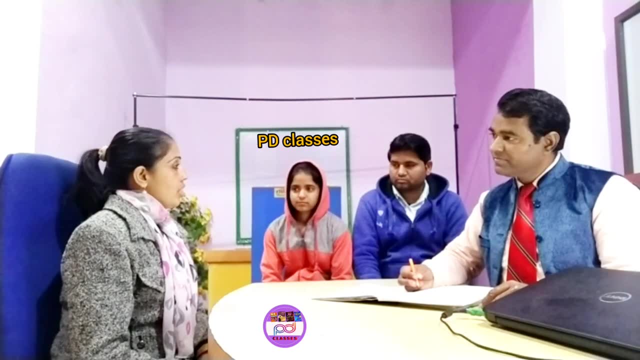 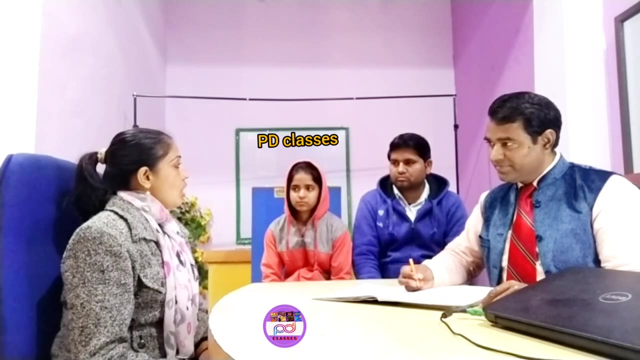 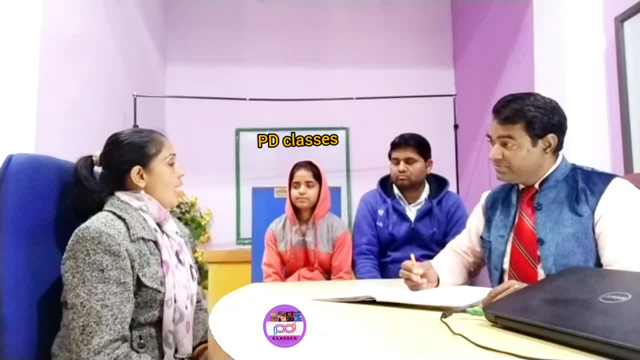 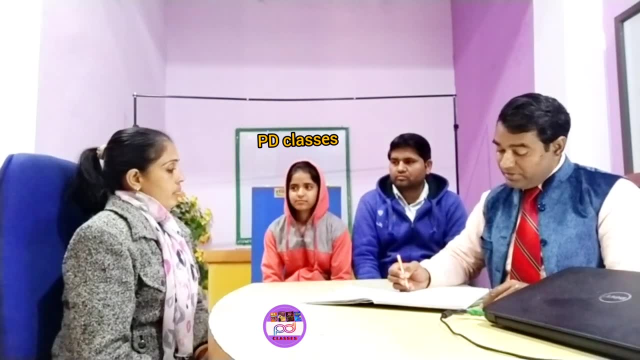 And I am a senior teacher. Yes, Thank you, I am good teacher. So am a good teacher. Yes, And May 15th of this year has I becoming another university architect- May 15th? yes, Yes, And am also a better teacher. Yes, I have got a job doing Class 11 on Monday. 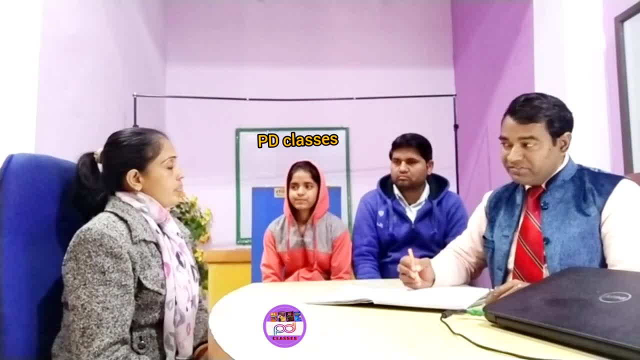 July 1st, Sagamshankala, Adi Madhavam. Yes, yes, yes. And now I am a seen professor at the Jit watt University of Money. I am also a graduated professor. the answer: yes, if the power of given number is in negative m. and we, then? we find the answer by: 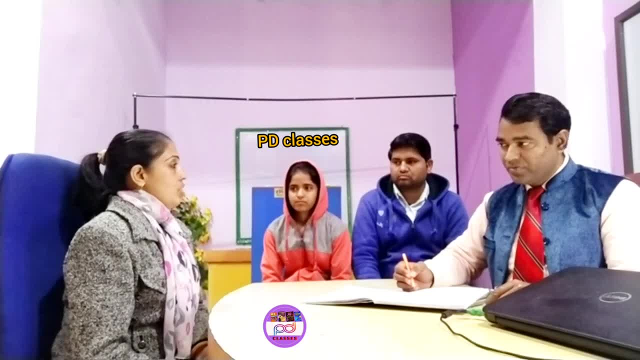 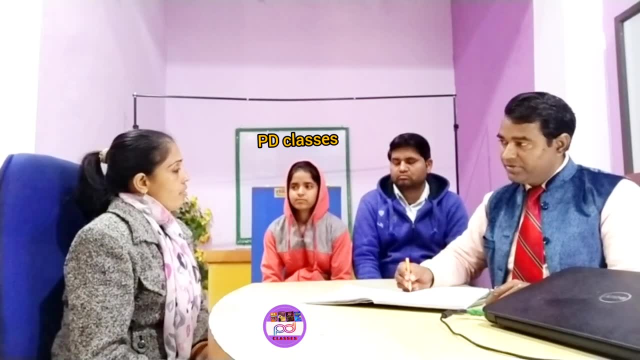 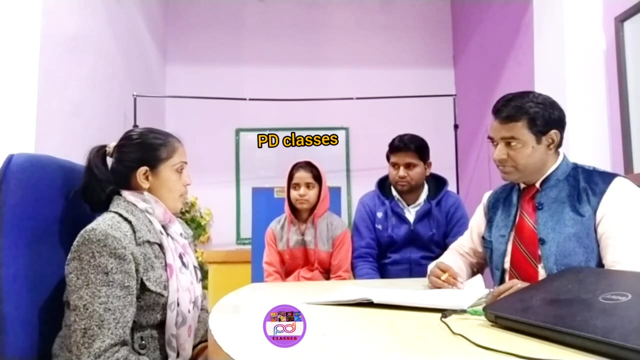 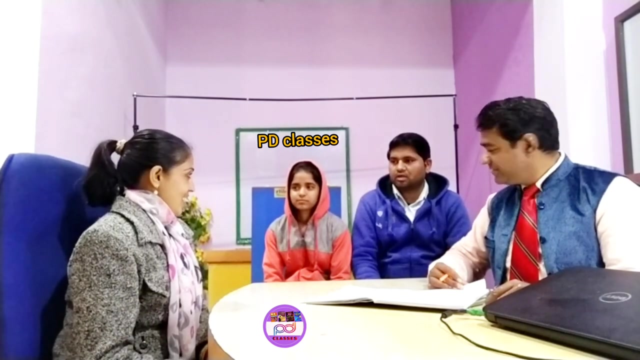 reciprocal, uh, the given number, like uh, three key power, uh, minus one. then we reciprocal one by three, then power is in positive form. the answer is one by three. okay, yes, please, mr anand, have your mathematical questions. so full form of lcm, lcm, lcm, full form, uh, yes, sorry, yes, so after a formula. 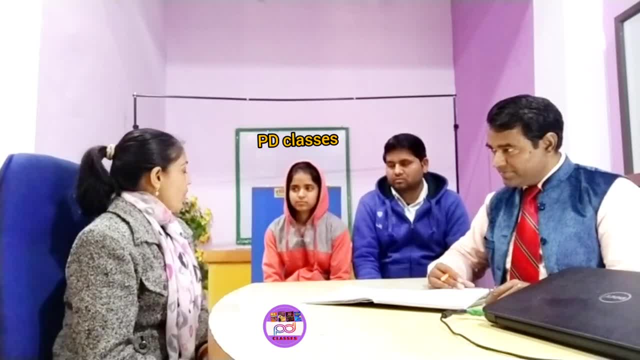 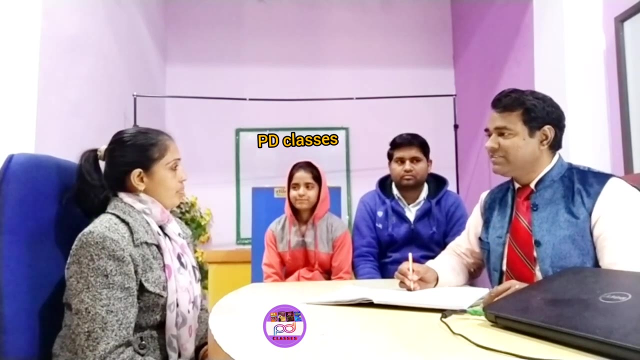 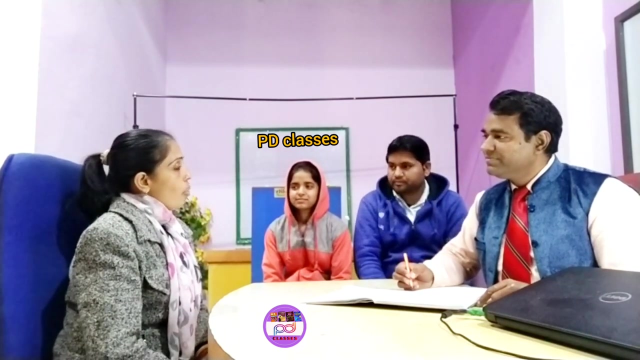 compound interest principal multiply by 1, plus rate divided by 100 and power equals to time minus principle. okay, suppose you have teacher, student the mathematics, and students are saying: madam, it is very tough subject, yes, so how will you put develop interest among your students? sir, it is a phobia between student that. 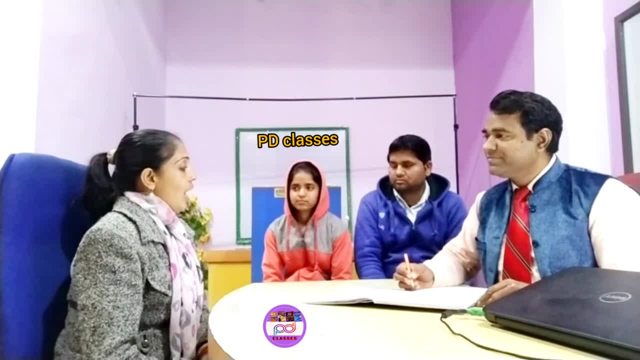 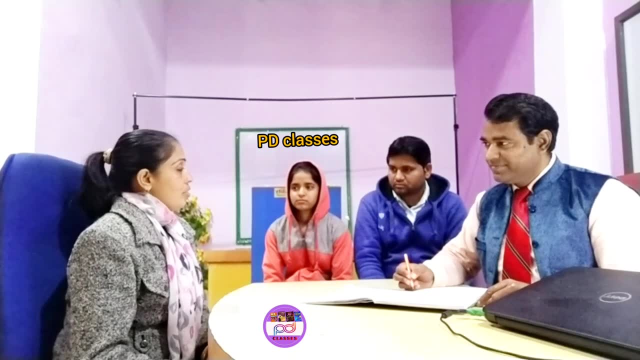 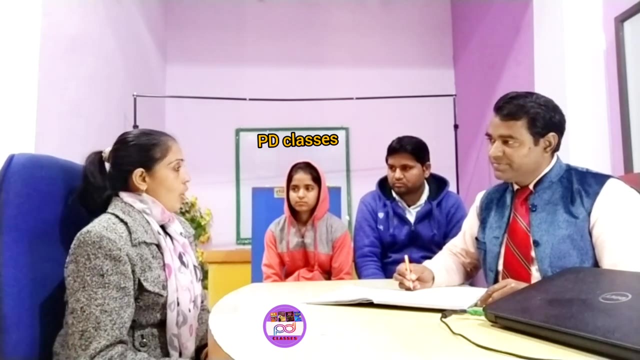 maths is a very difficult subject, right, but i think math is really very easy. if we understood their concept, then there is no fear about this. so i try my best to understood the student, their concept, and, okay, you make it intelligent. yes, sir, suppose this is your first class in a 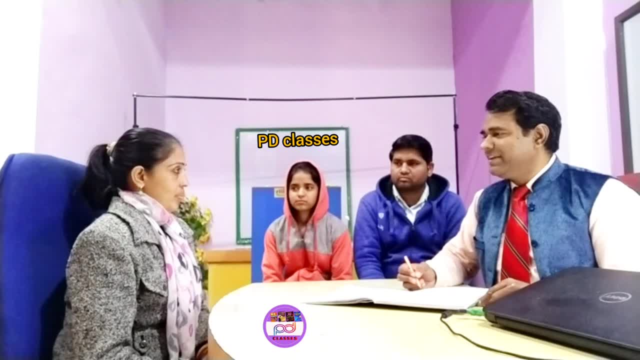 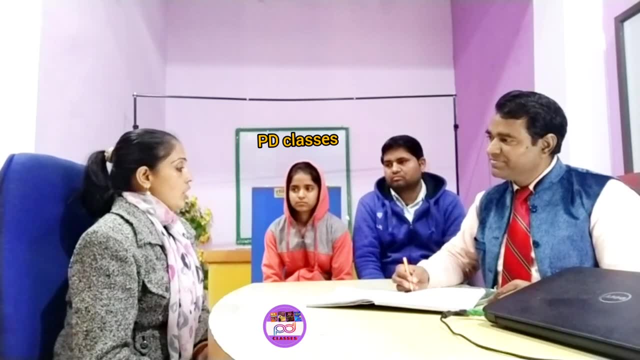 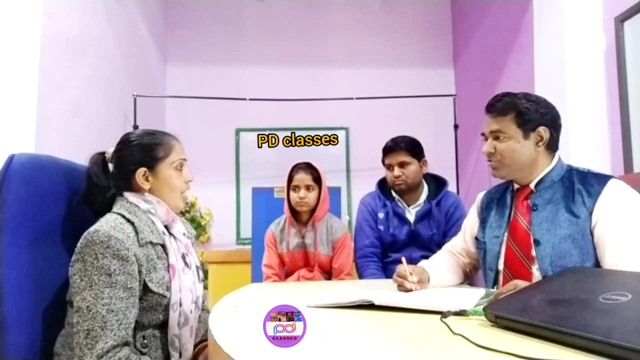 class and you are going in your class, so which topic you will take initially? okay, sir, first of all, uh, in first class student, i will teach them adding okay, okay, without any, using a paper, pen or blackboard. so suppose we are the students? yes, and you have to. 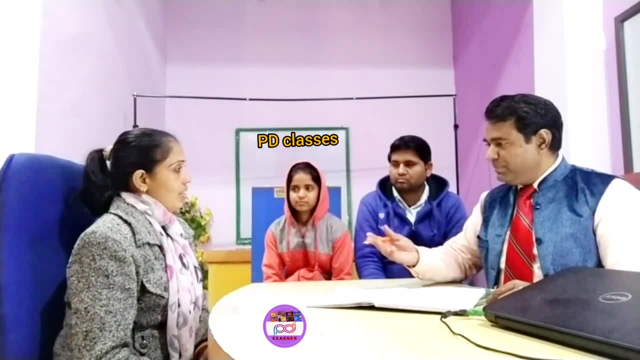 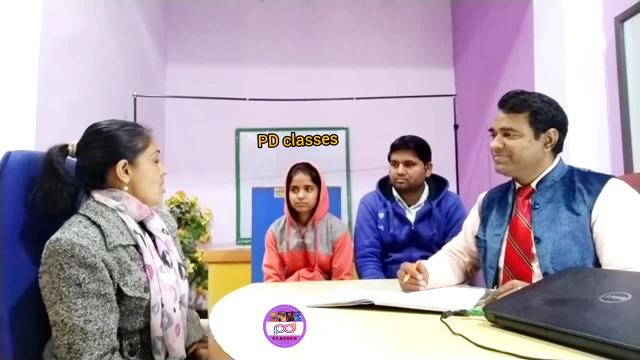 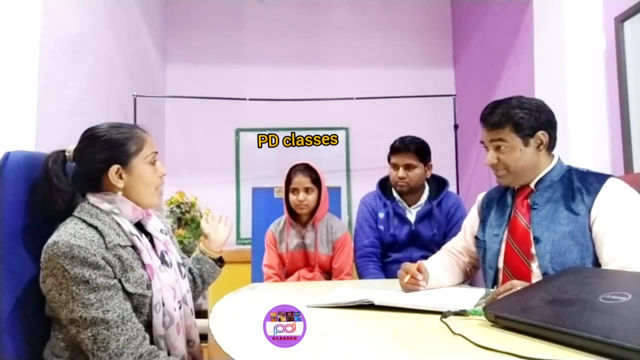 give your demo on adding yeah and this is the first class. yeah, sir, please give your demo. yes, sir, students, first i stand up and to stand as two students and then in third student. i will ask now how many students are standing in front of me, okay, uh, these students easily tell that there are. 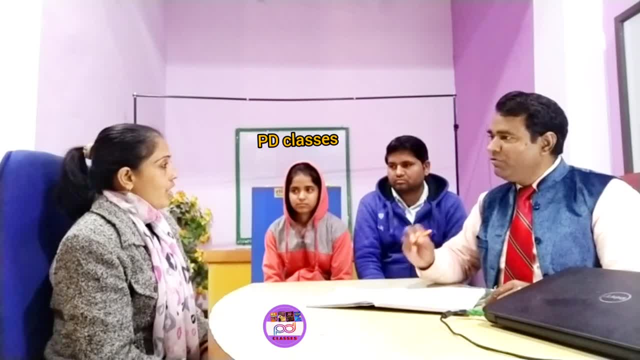 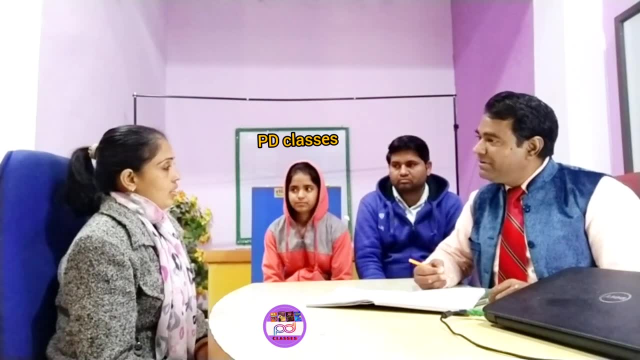 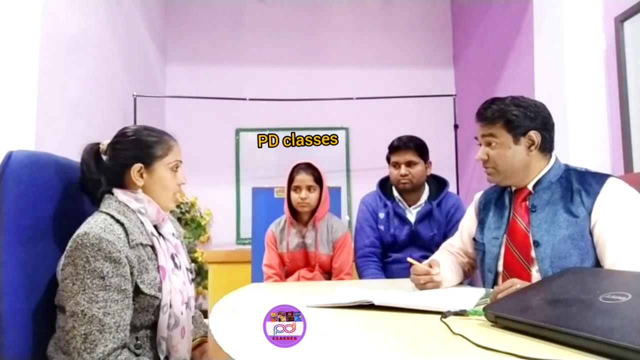 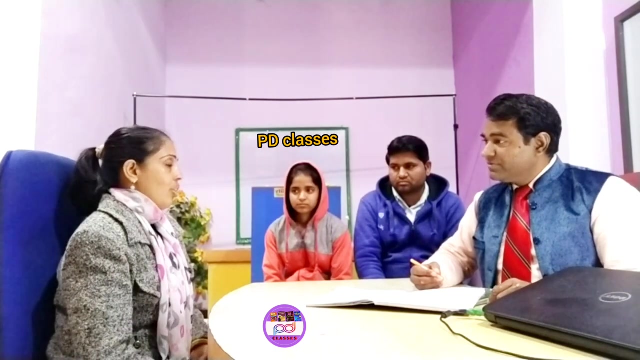 two students right, yes, sir, so in this way, add the things. okay, he has done the addition. yes sir, yes sir. okay, then how multiply will be done with any example. multiply is doing by. yes, yeah, you must be able first of all. i learned about tables without table multiplies, not okay, so first you will teach. 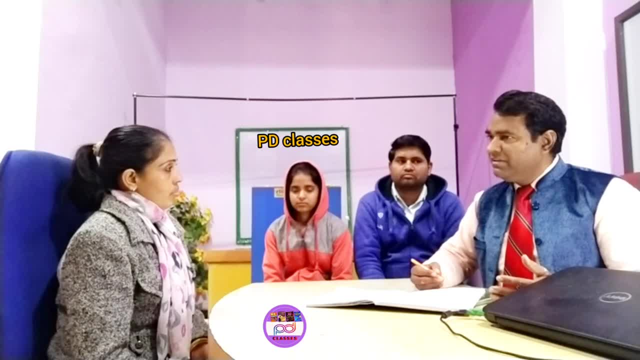 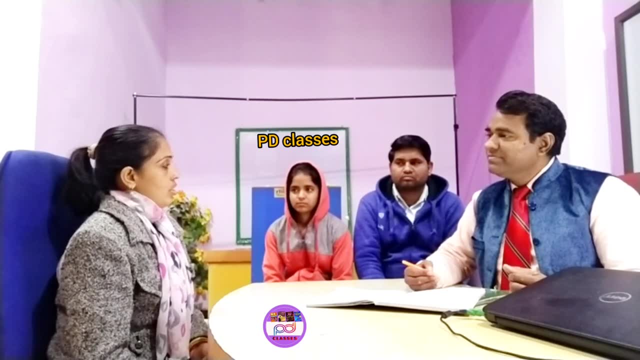 your students about the tables? yes, sir, but you know table cramming is i don't think it is a good habit. so what is your way to teach them tables? what is the best way? yes, sir, teach them how you make them teach this learning tables easily. is there any way? yeah, 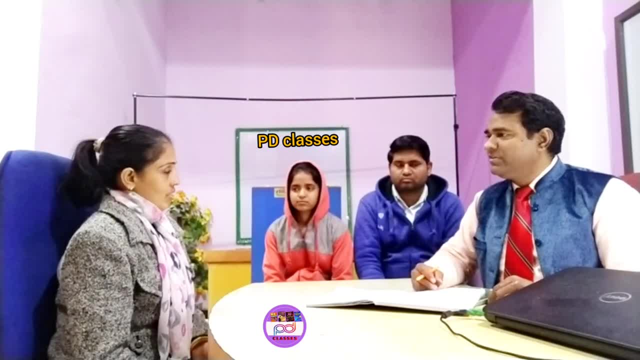 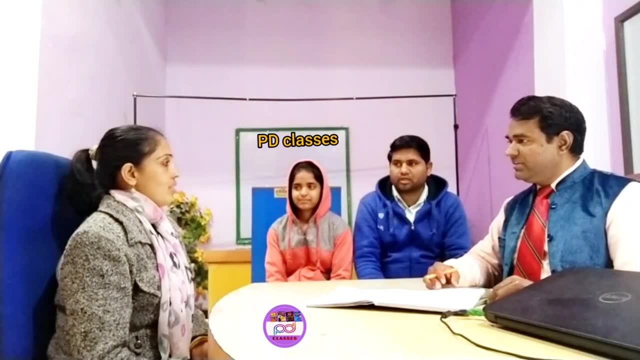 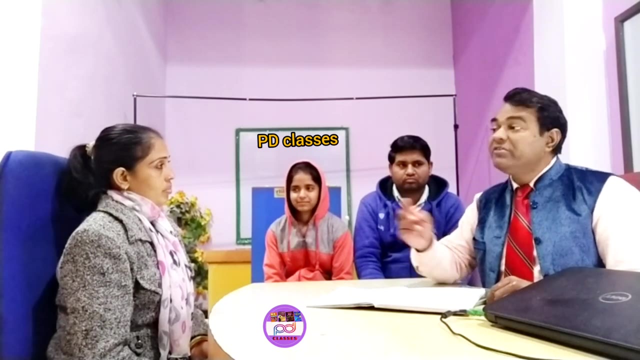 no, okay, but since you are handling only prd and small students, so you need not such good tricks, you require but when you go with upper classes, definitely the time short is. yes, yes, yes, yes, yes. so can you tell me what are the best qualities you are having out of the qualities? 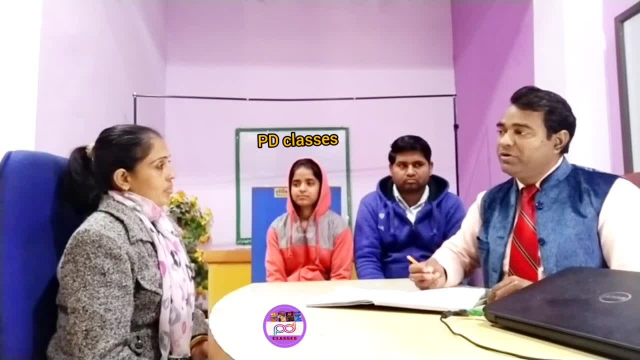 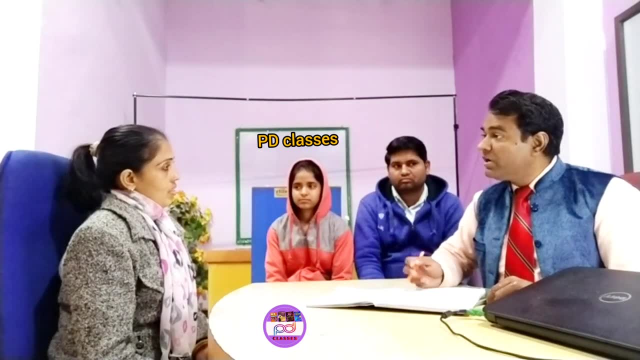 you just now told me which quality you are having to be a good teacher. yes, sir, i'm a good listener. okay, i have a good command on my subject. but, ritu, we have so many girls- those who are standing in a queue like you, yes, and they are also going for the same job. 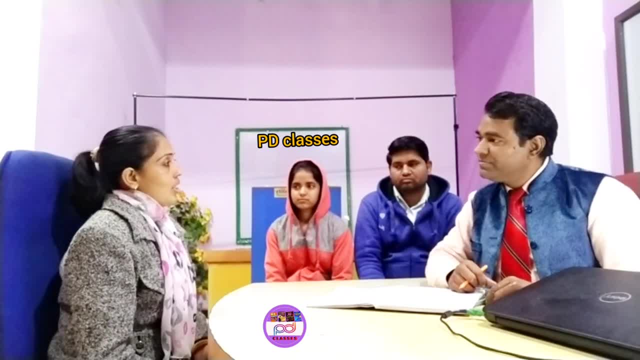 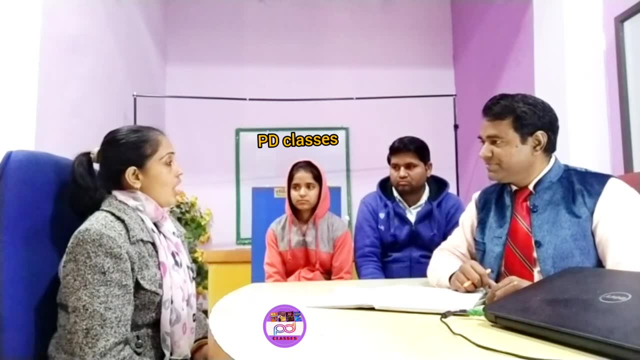 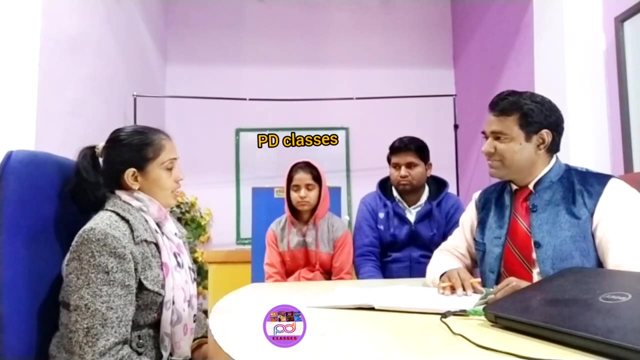 then why shouldn't i recruit them rather than you? yes, sir, sir, i have a solubrious experience which will be definitely fruitful for our exam organizations. okay, and i'm a versatile so i can adjust anywhere. so that are the qualities, okay, which makes you different from us, see, in this job. 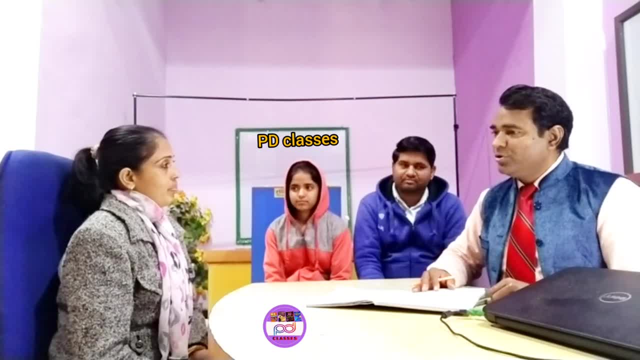 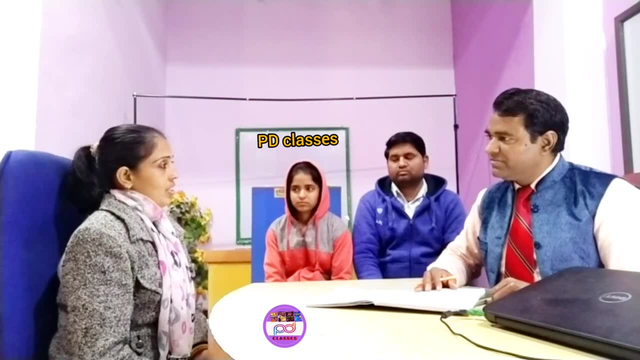 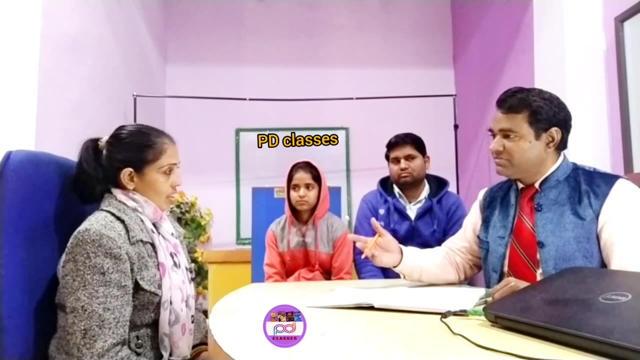 this is a very disciplined organization. so you know, here you have to be punctual every time and you have to be a committed personality. so how will you manage all these things, sir? i will you have a baby also? yes, so how will you manage your- uh, baby girl and all these things with your family? yes, 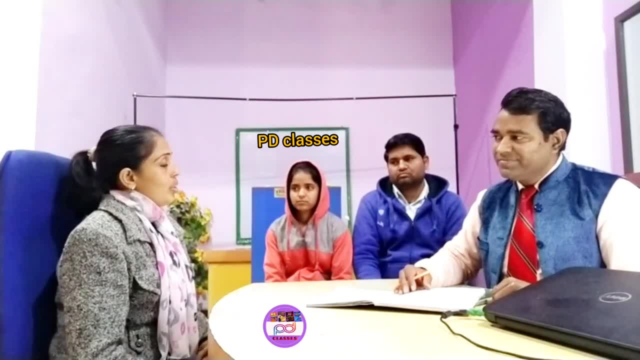 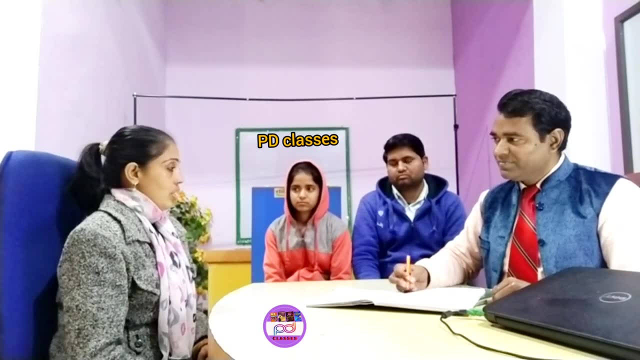 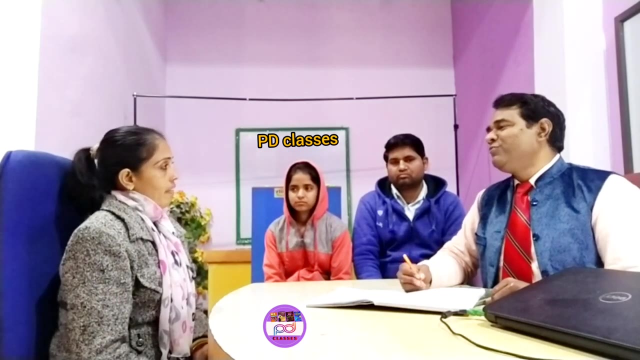 doing job, don't you think it would be a hectic for you? no, sir, because the teaching is my passion, it is my hobby, so it is not uh tough for me for handle. uh, my family is very supportive, so i don't have any. okay, my very important question from you is what? 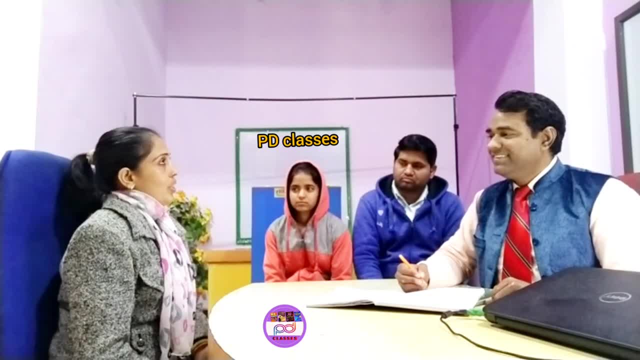 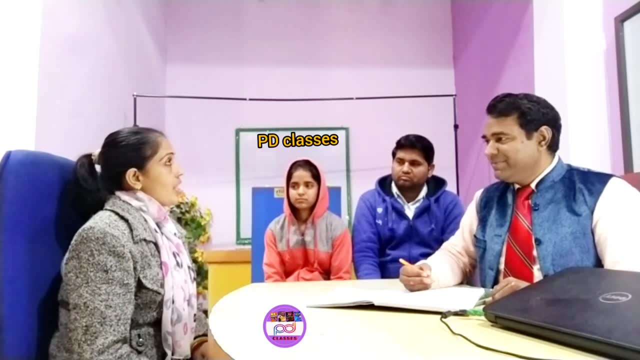 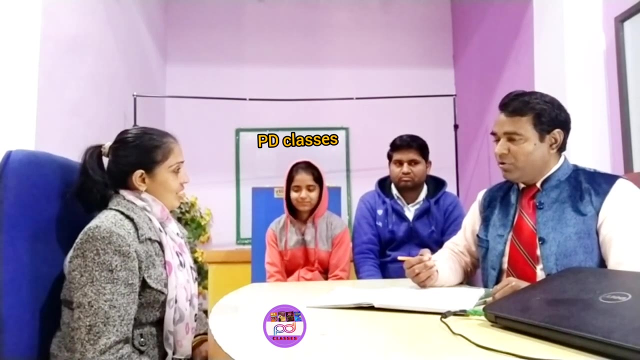 is your weakness, sir? okay, uh, do you think anytime? uh, what can be my weakness? can be very weakness, sir. my weakness is that i easily believe anyone. oh, so you believe more others. yeah, although it is good, because without faith we can't do anything but too much of believing or easily believable. 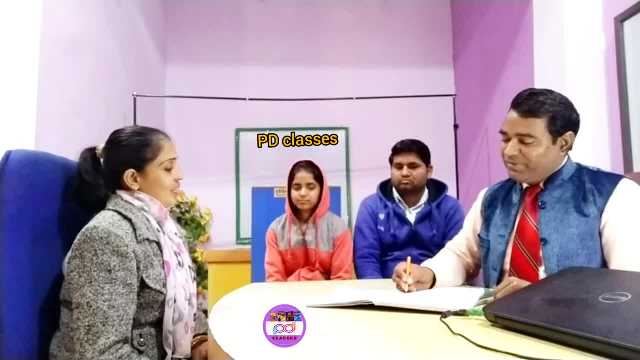 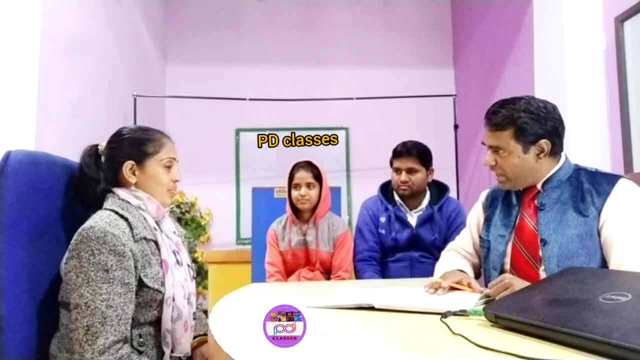 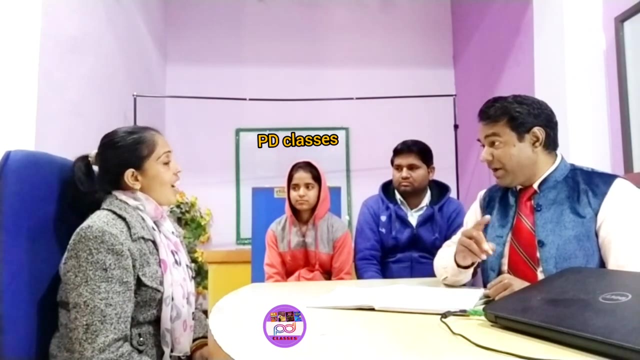 is a big risk also. yes, sir, okay. so students might also take benefit out of a teacher. yes, yes, okay. so although the interview was first session with you mathematics questions, we have given good answers. okay, so go through the topics and uh, lcm at scf. yes, the full forms can be asked in the largest. 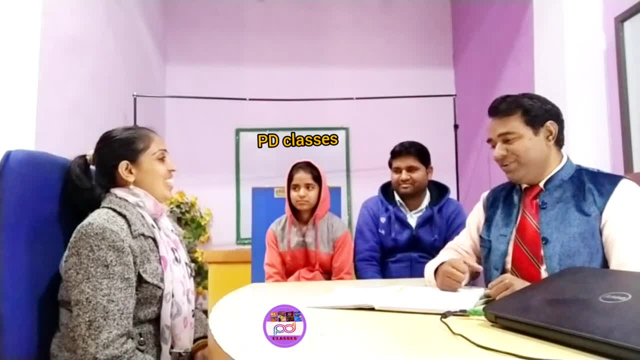 common factor. okay, now you recall the answer. yes, very good, very good, we are proud of you, thank you.